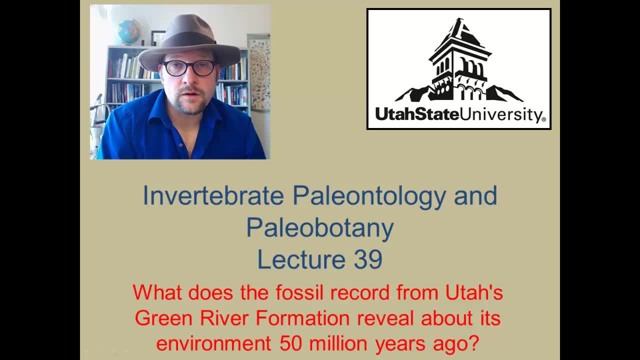 Welcome to Utah State University's Invertebrate Paleontology and Paleobotany class. This is lecture 39, where we will look at a local fossil site here in Utah, the famous Green River Formation, and examine the fossil flora. We will use these fossils to reconstruct the 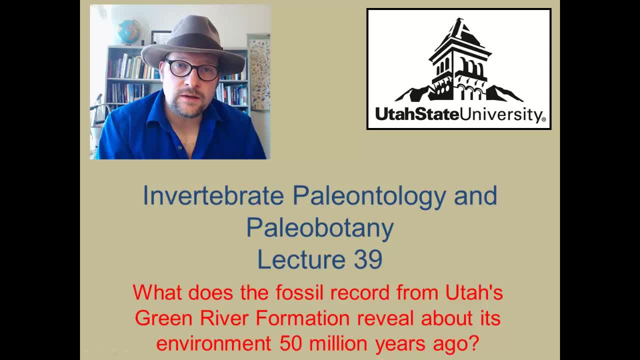 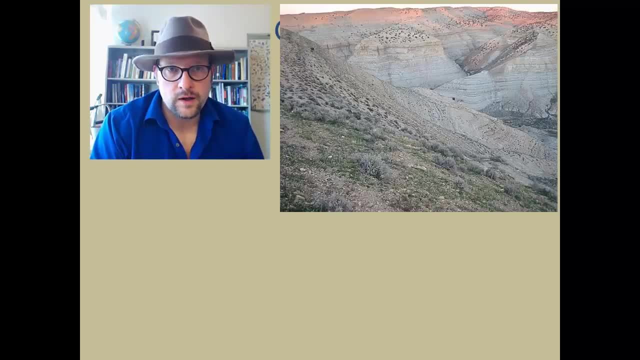 environment 50 million years ago during the Middle Eocene. in North America, The Green River Formation is exposed in the Tri-State region of Utah, Wyoming and western Colorado. The Green River Formation is a layer of thickly stacked shales and sandstones exposed. 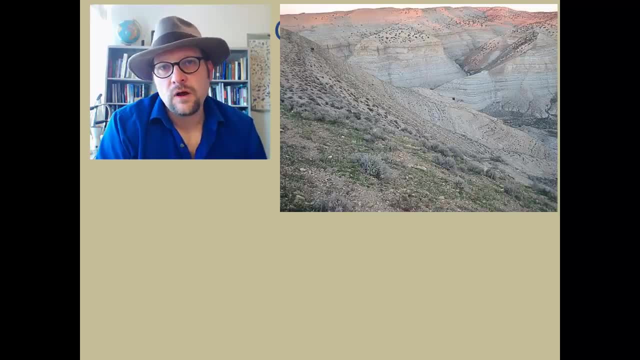 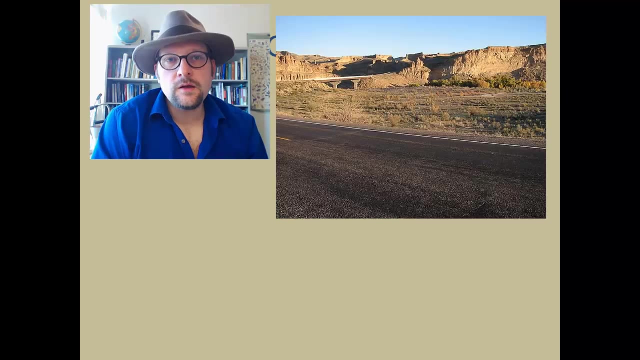 throughout the canyonlands of northeastern Utah, western Colorado, as well as a region near the type section in Green River, Wyoming. One of the most famous fossil sites here in Utah is the Cowboy Canyon area, which is along the drainage of the White River Here in Utah. the lower and upper portions of the formation are composed of thick sandstones. 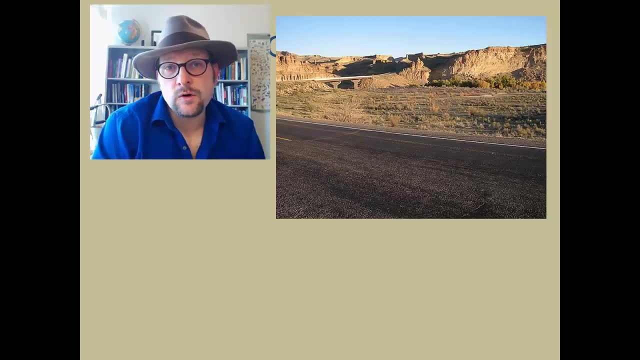 The more coarse sandy grains reflect a more fluvial or groups of rivers, while the middle shale interval are finer grained muds and these reflect a lacustrine or lake deposits. It is in these lake deposits that we find most of the fossils The lacustrine faces 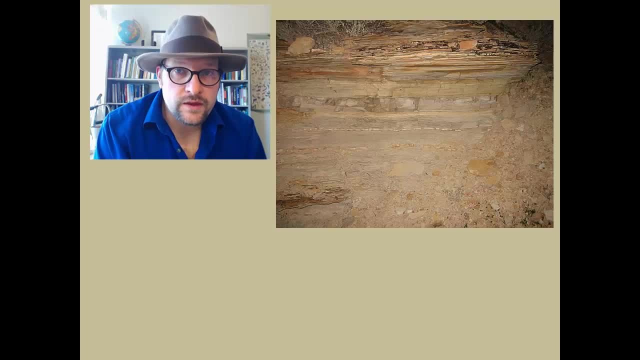 of the Green River Formation are stacked like this. There are several layers of thin shales which contain an abundance of fossils. The trick in excavating them out is to dig down and then split the shale along the face to expose the hidden fossils. There are a number of public and private quarries that exist that 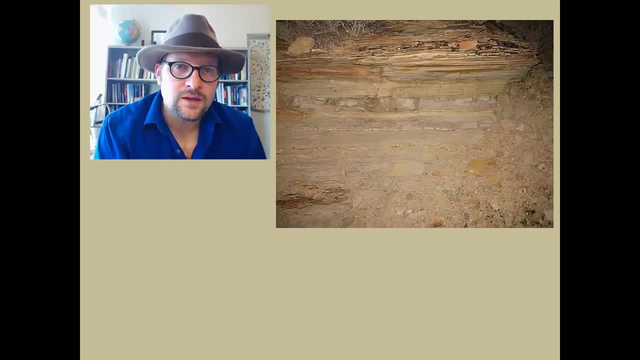 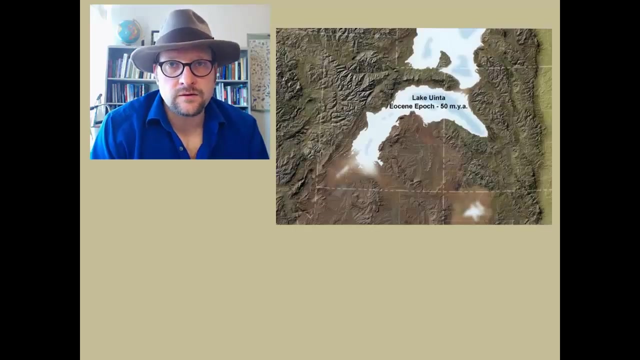 allow you to collect fossil plants in the region. The real key to finding fossil leaves is to expose those layers which are buried in thick pages of sediment. It is a bit like a giant book that is filled with fossils on each page. The Green River Formation represents a thick lake system that existed in the area during. 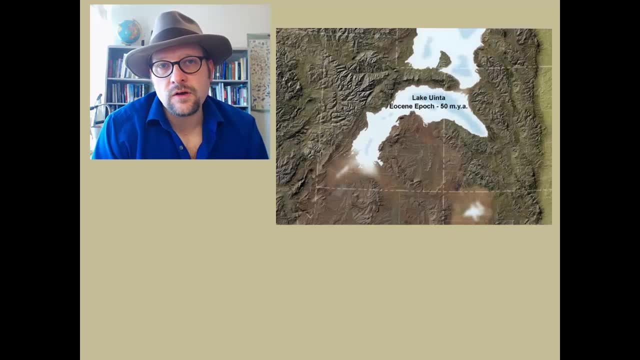 the Middle Eocene. The southern ancient lake is called Lake Uinta, while the northern lake is called Lake Goshute. Near the severe thrust of western Wyoming was a separate lake that is not depicted on this map. that may have been isolated from other lakes called Fossil. 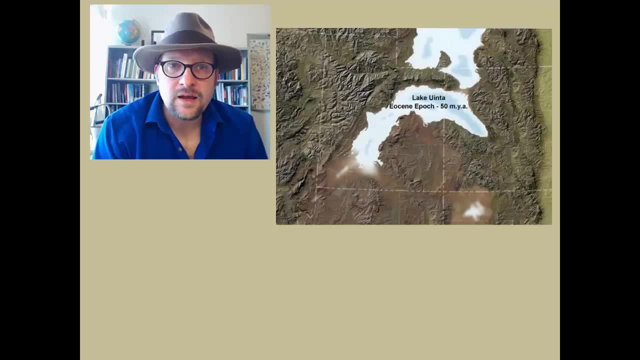 Lake. These lakes were never very deep and they are not as big as the Great Lakes that exist today in the northeastern part of the United States. They are about a tenth of the size of the Black Sea in Eurasia, so they are a moderately 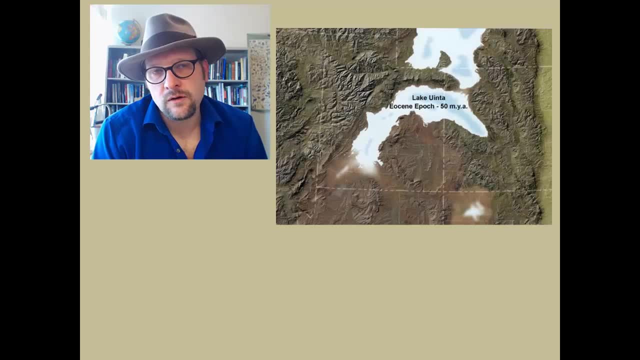 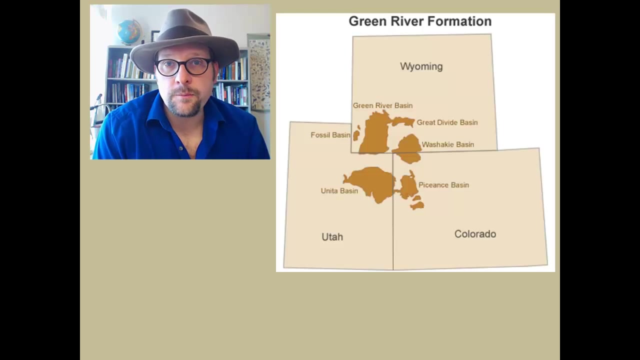 large lake system, but there are many larger lake systems of the world today. The lake system is much older than the Pleistocene Lake Bonneville, which was an expansion of the Great Salt Lake in western Utah during the Ice Ages. Today, the region is divided up into a number of basins surrounded by high mountain ranges. 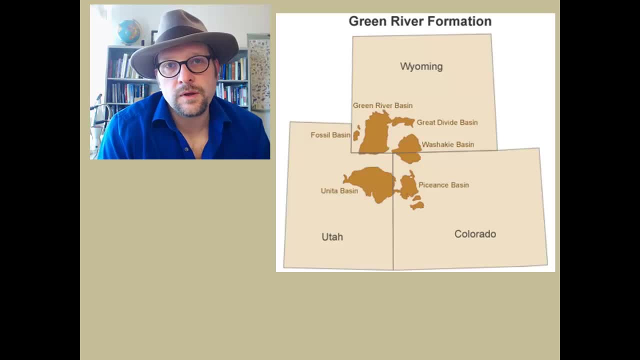 including the Uinta Basin in Utah, the Piance River Basin and the Lake Uinta Basin in Utah, The Piance Creek Basin in western Colorado and the Washakie Basin of southern Wyoming and the Great Divide Basin and Greater Green River Basins and Fossil Basin of southwest 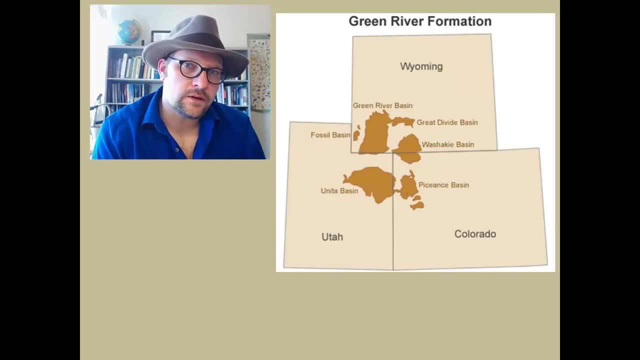 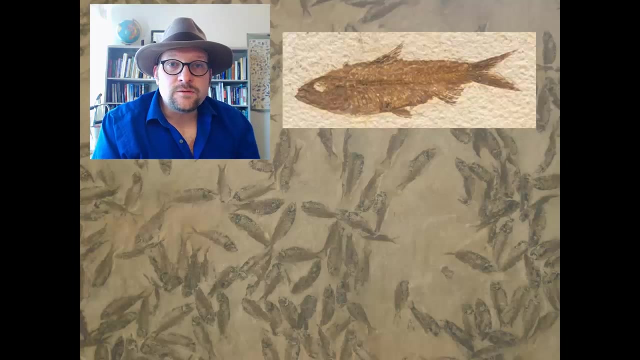 Wyoming. Each basin preserves sediments of these lakes that existed during the Eocene. These lakes were often flooding back and forth across the landscape, leaving behind a record today of animals and plants that fell into these shallow lakes. The Green River Formation is known for its incredible fossil fish, including the state fossil of Wyoming Nidia, which is 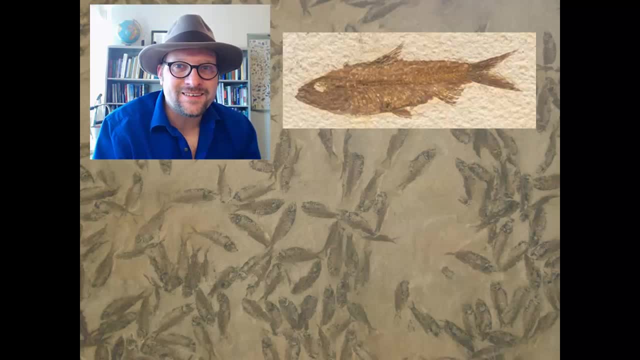 a little fish that is related to modern sardines. These fish lived in large schools and likely died en masse during periods of temperature and chemical changes in the lake systems. They are very common as fossils and they likely formed these giant schools of fish. 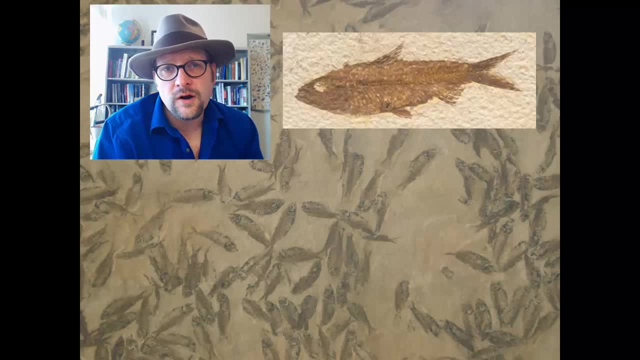 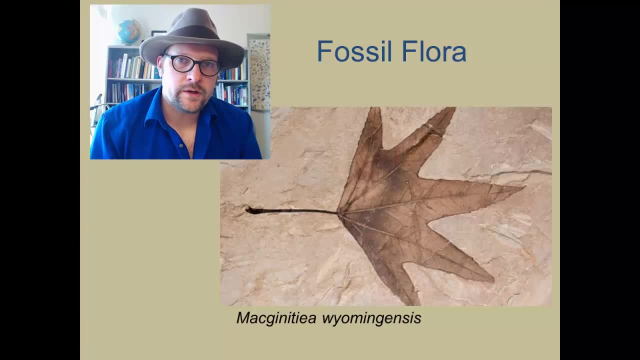 numbering in the millions. They provided food for other fish known from the formation, as well as for shore bird fauna. Today, we are going to talk about the fossil plants from the Green River Formation and use that information to reconstruct what eastern Utah may have looked like 50 million years. 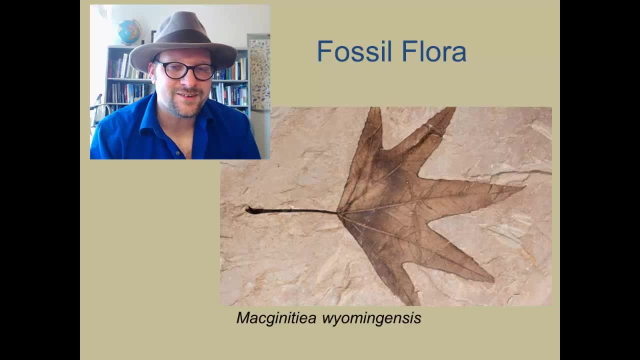 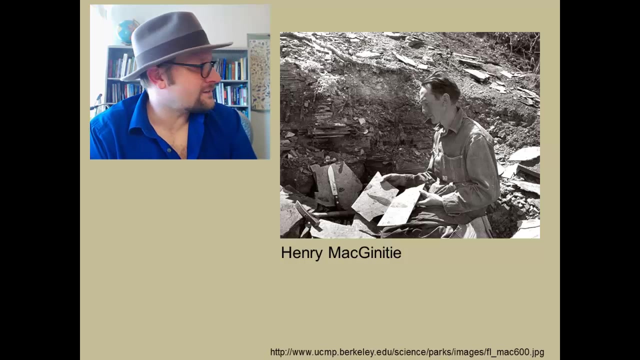 ago. The first and likely most characteristic fossil leaf of the Green River Formation is the fossil McGinneyi. It is very characteristic with its multi-pronged leaf margins. McGinneyi was named after the American paleontologist Henry McGinney, shown here collecting fossil. 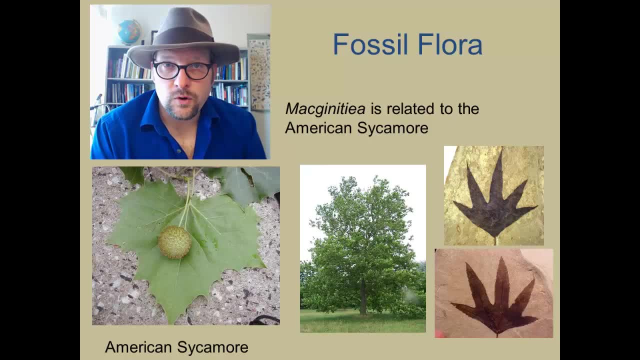 leaves McGinneyi is related to the American sycamore tree, which today only lives in the eastern United States. The occurrence of this relative throughout the western part of North America during the Eocene indicates a much warmer and more temperate climate during the Eocene. 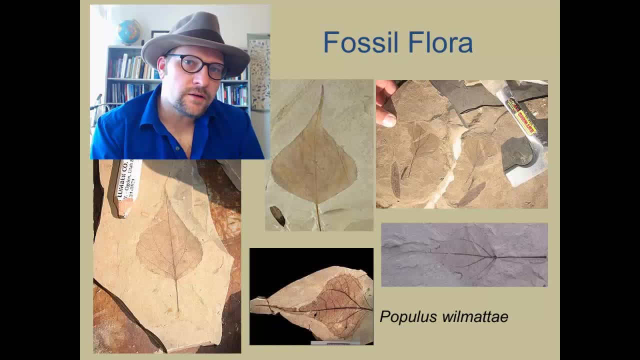 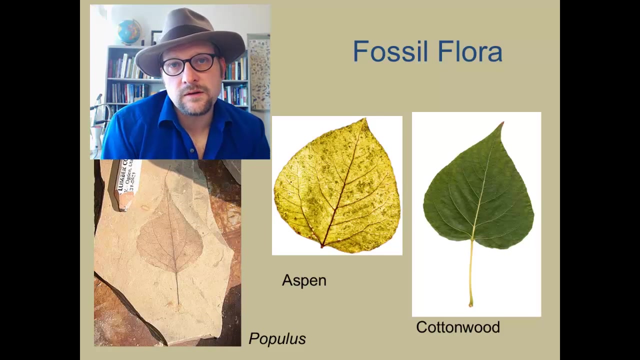 for Utah, Wyoming and Colorado. One of the most common fossil leaves in the Green River Formation is Populus wilmadi with a very characteristic leaf. I have found a few of these specimens myself, splitting them apart. Populus is a very specious plant with a number of living species, including both the cottonwood 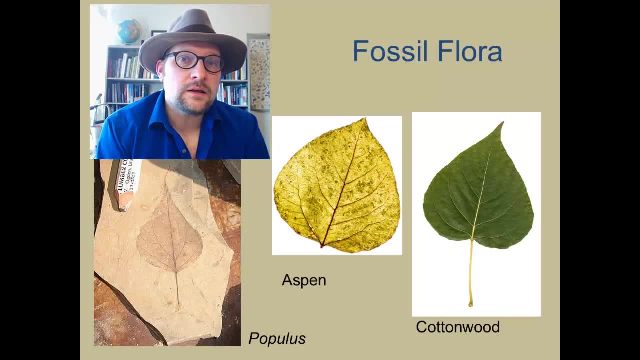 and aspen trees native to Utah. It is likely that this Eocene species was more similar to some of the living poplars and common along the banks of this lake system. Another fairly common fossil plant is a variety of fossil legumes, likely members of the family. 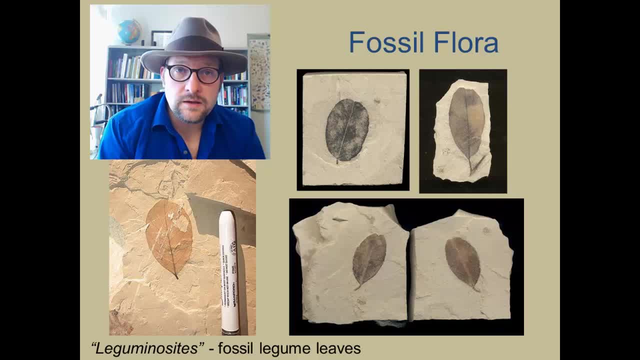 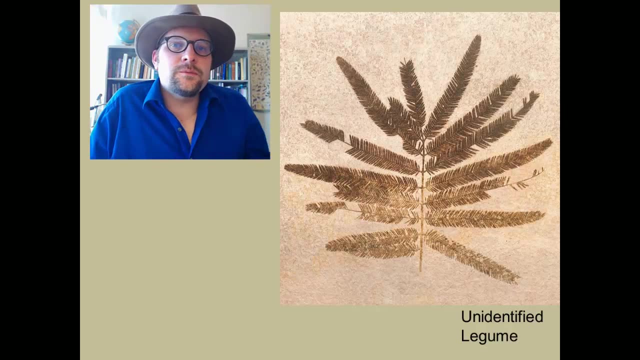 Fabrycia. This is the group that includes peas, beans and lentils and is likely a source of food for the diverse birds and mammals known from the Green River Formation. This is not a fern. it is an unidentified legume, and many legumes have multiple leaves. 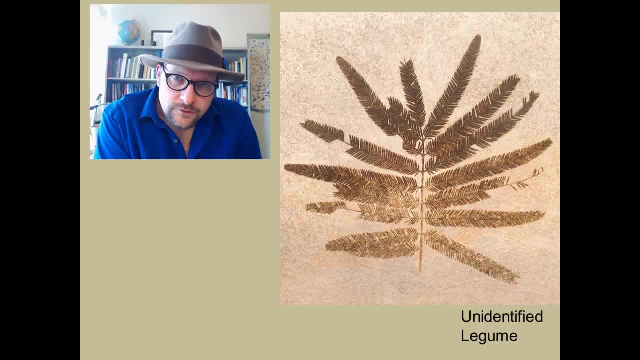 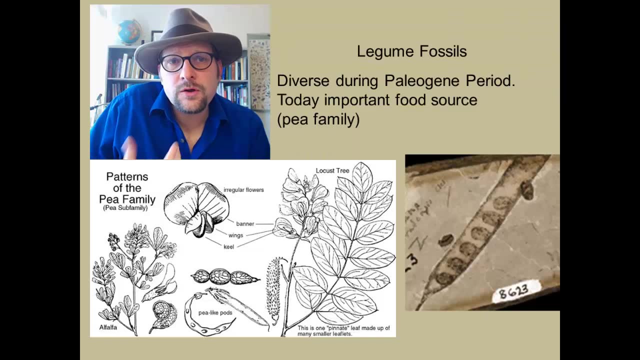 like this very cool specimen. True ferns are also known from the Green River Formation, but are rare, and their appearance indicates a wet and warm climate. Legumes are interesting because they serve as an important food source for the mammals living at that time and during. 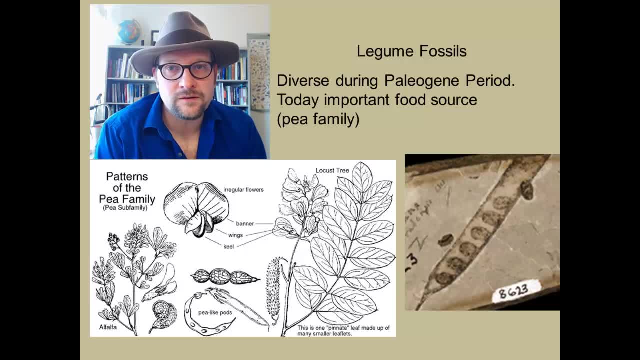 the Green River Formation's deposition. there were numerous species of primates here in North America- lemur-like primates and nocturnal tarsier-like primates, which likely relied on these food sources or the insects that fed on these plants. 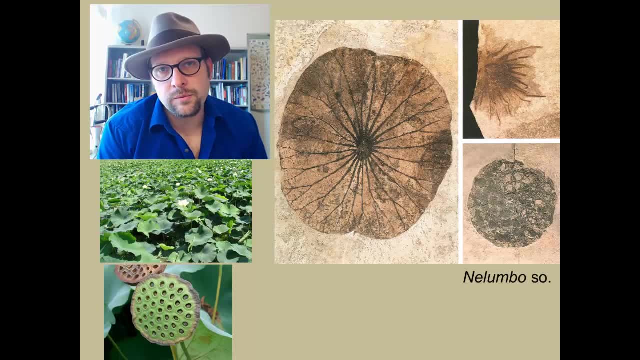 Being close to a large lake system, there are many water plants, such as the locust plant, which is distantly related to water lilies. It is placed in the Eudicots, but is found in ponds and lakes in tropical regions today. 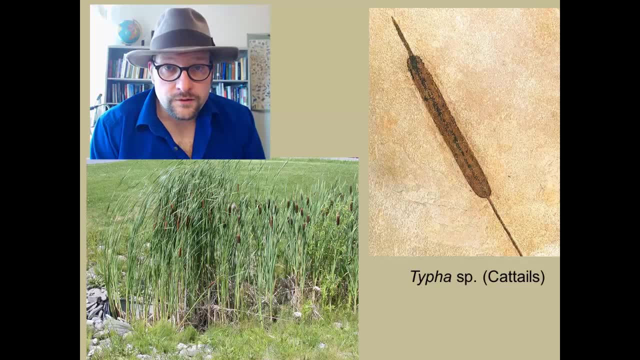 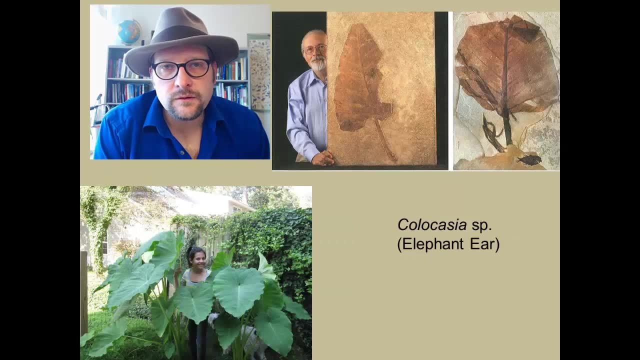 Cactails have been found, as well as horsetails, both found in wetlands today and are found in the Green River Formation as well. Another remarkable fossil is the large leaves of Coleaceae. This is the elephant ear plant. 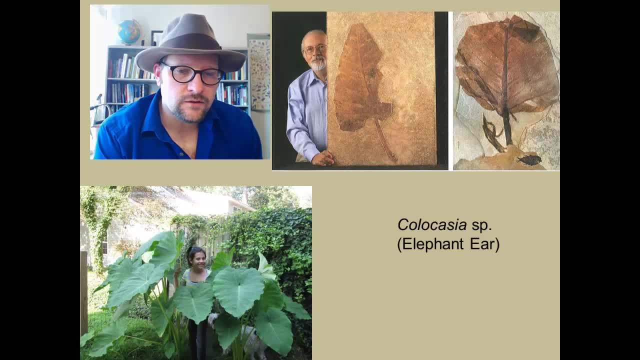 which is native to southeastern Asia. Today it is an invasive plant in Florida, where it grows in the warm, tropical, wet climate of that state. The presence of the fossil in Utah and Wyoming harks to a really wet and tropical past, and it is believed to have 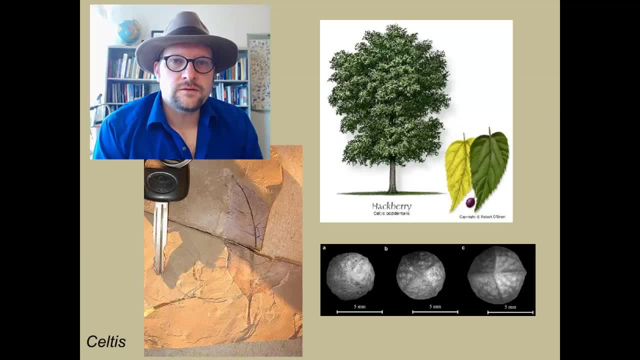 been found in the Eocene for Utah and Wyoming. Another fossil is the Sutleus. This is the hackleberry tree, which is found in many Eocene sites in the Rocky Mountains. It is a smaller tree with serrated leaves and smaller seeds. 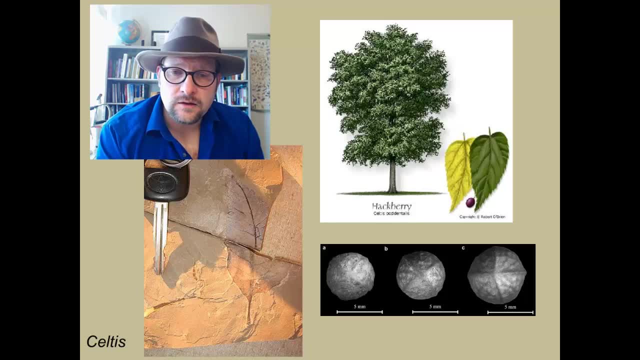 that easily preserve as fossils. They grow today in Utah and are often found in urban settings, where they are planted because they are drought tolerant. It is rather rare in the Green River Formation to find these, but it is more common in some of the upland environments. 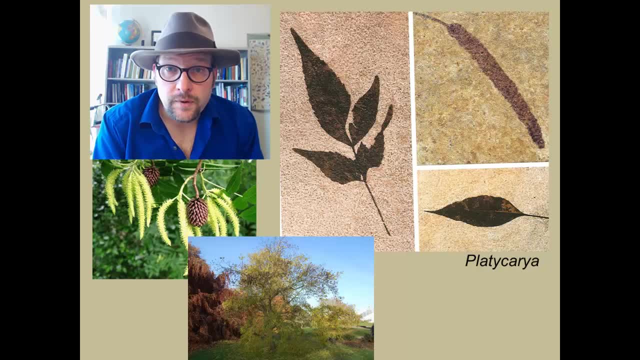 One of the most common fossil leaves in the Green River Formation is the genus Platycaria. Today it lives in Asia, in particular in China, Korea and Japan. It is a member of the walnut family and it has long female catkins bundles of flowers. The seeds are spiky cone like. 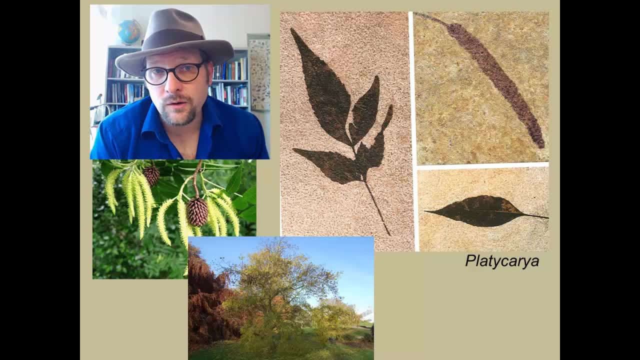 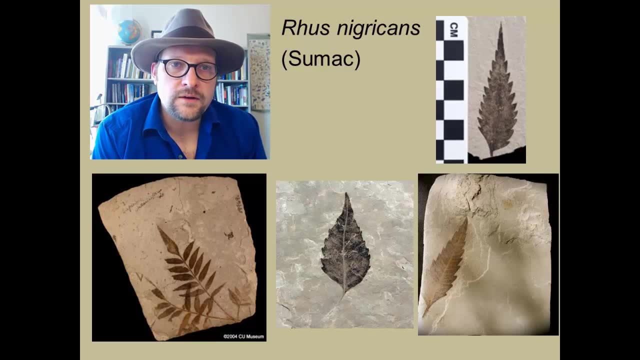 structures which are often mistaken as conifer pine cones. The next common fossil leaf in the Green River Formation is Rudeus nicarius, which is sumac. They have these toothed slender leaves and I found a number of these as well in the Green. 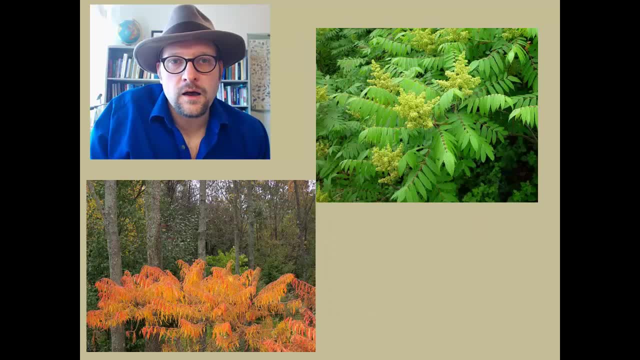 River Formation. Today, sumac grows in Utah and in fact there are a number of sumac that live along the canals, creeks and foothills of the Uintah Mountains in Vernal. The leaves show these fantastic bright colors. in the autumn, The Green River fossils are placed. 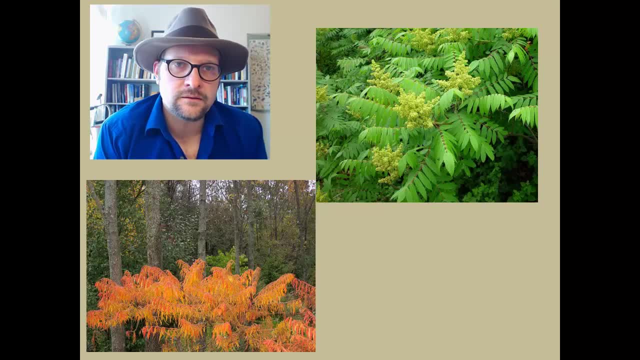 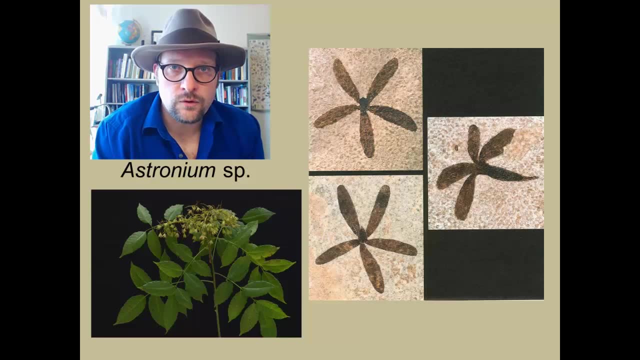 in a separate species, but the genus is a pretty specious plant and there are species known in North America, Asia and Europe. Fossil flowers are known of the genus Astrodium, which is a member of the cashew trees. It 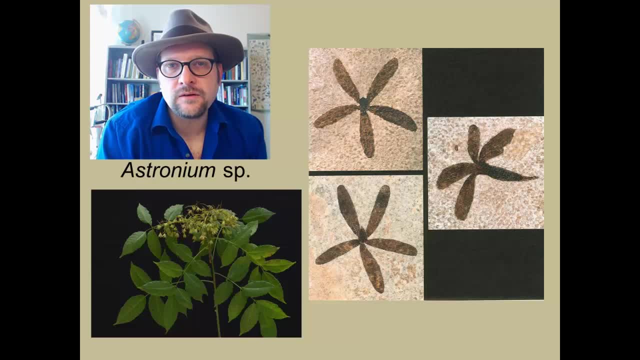 is native to Central and South America, with many species living in Brazil. The presence in Utah and Wyoming demonstrates a much warmer environment during the Eocene. In fact, there are a number of invertebrates and other plants today that are restricted to Central and South. 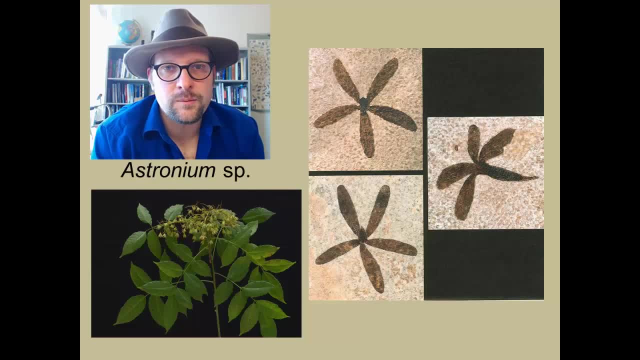 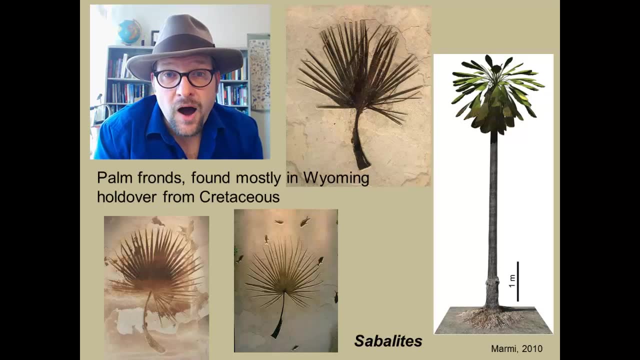 America, but during the Eocene they had ranges all the way up into Northern Wyoming. Most striking in terms of how warm it was during the Eocene is the discovery of fossil palm fronds placed in the genus Scabalates. Palms only grow today in places which rarely get. 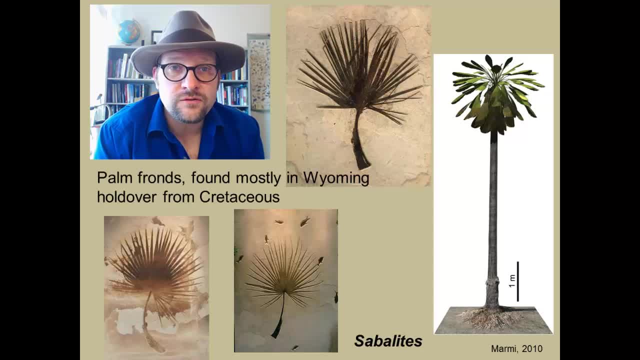 below freezing temperatures and the presence of palm fronds in Wyoming during the Eocene strongly indicates that it was a much warmer and wetter environment during the Middle Eocene. Date palms have also been reported from the Green River Formation, which today grow in. 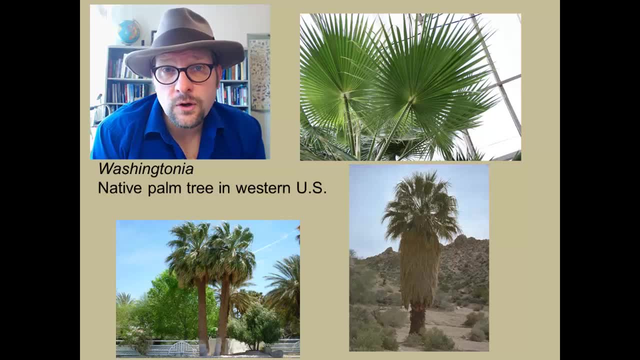 Southeast Asia. Scabalates is closely related to Washitonia, which is a native plant tree in the Southwestern United States. It grows today mostly in California, Arizona and can be found growing in Southern Utah. It is fairly tolerant of cold temperatures but does not. 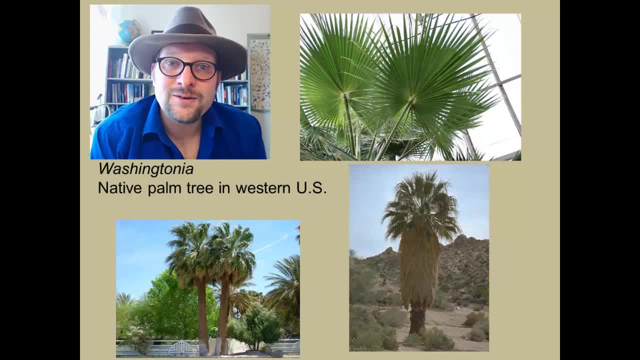 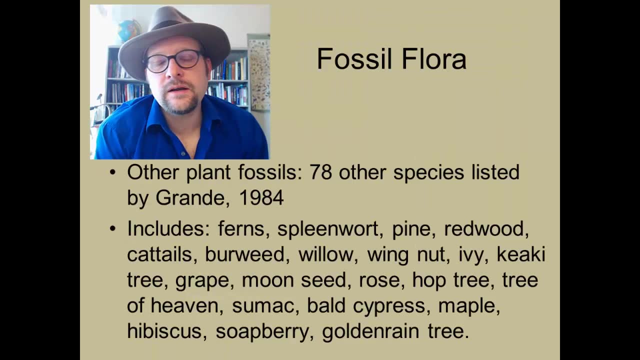 grow in Colorado, Northern Utah or Wyoming today. During the Eocene its range expanded north into Wyoming, although these fossils are placed in a different genus. Lance Grandy's 1984 book lists 78 species of scabalates, including the Scabalates as. 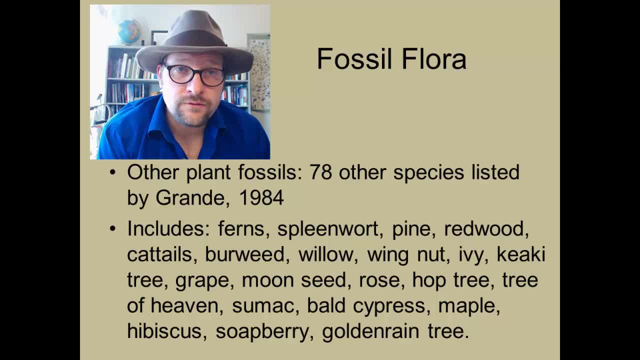 well as several species of fossil plants from the Green River Formation, including ferns, splee, warts, pines, redwoods, cottontails, burrweed, willow, wingnut, ivory, kiki trees, grapes, moon seeds, roses, hop trees, tree of heaven, sumacs, bald cypress, maples, hibiscus. 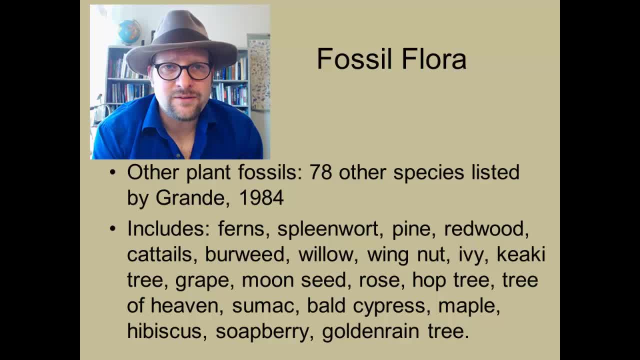 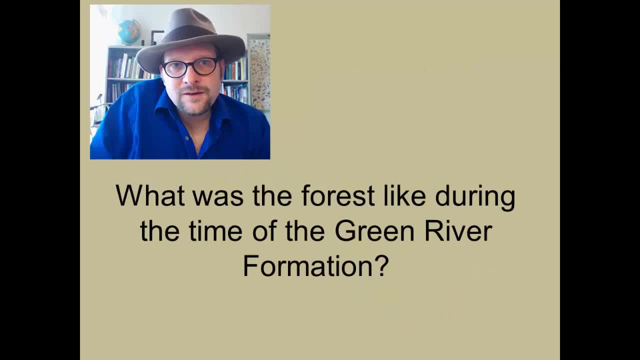 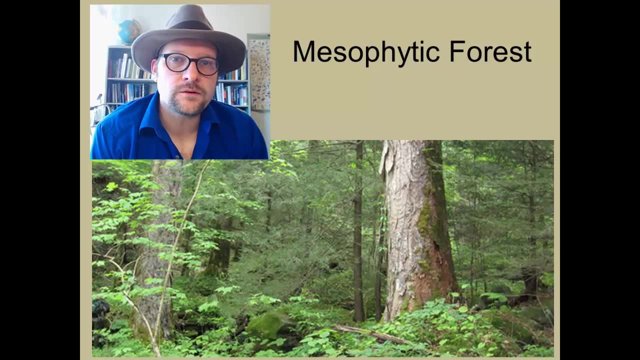 soapberry, golden rain trees and guava. So we have a diverse flora from the Green River Formation, which is continually being expanded with new discoveries. So what was the forest like During the time of the Green River Formation? most paleontologists reconstruct the forests. 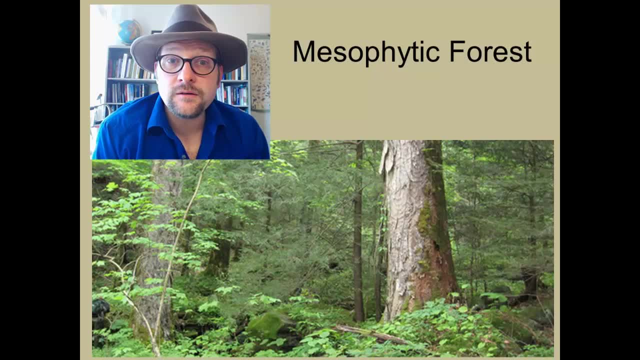 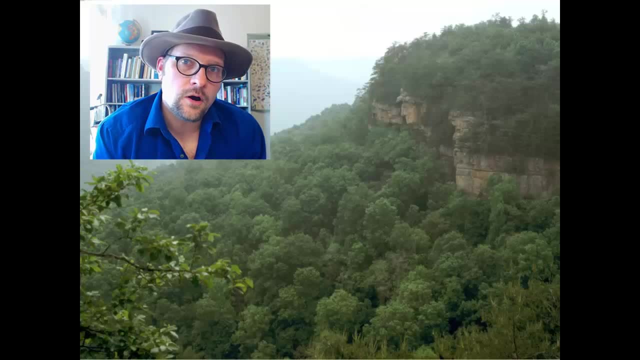 of eastern Utah, Wyoming and western Colorado as a mesophilic forest, something like what we find in Alabama today or even Florida. It was likely a dense forest with many large hardwood trees and a mix of conifer and some palms growing. 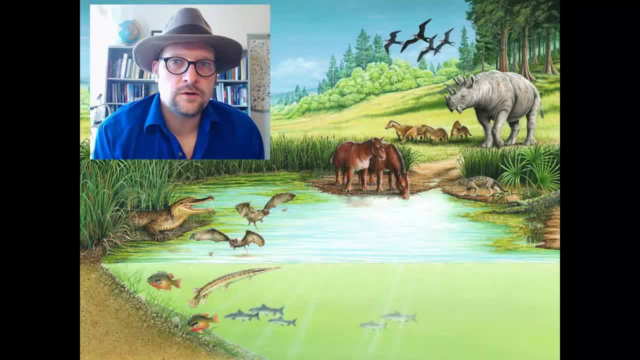 So let's take a look at some of the reconstructions made of the Eocene here in Utah, which was also a time period of many strange mammals like the multi-horned and sage-eared eocene. The Eocene was a time period of many strange mammals like the multi-horned and sage-eared. 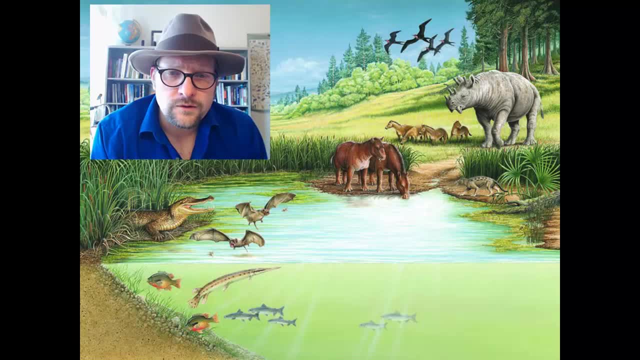 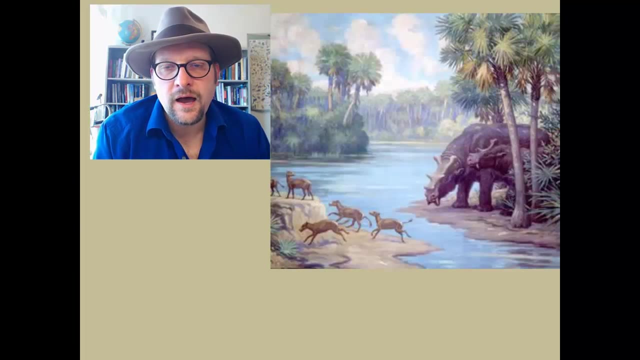 eocene: early horned and sabertooth euenithyrs, early horses like Orahippus and Protohippus, the oldest bats and unique fossil birds, turtles and crocodilians, as well as numerous fossil fish. This is another older reconstruction of the Eocene highlighting palm trees. 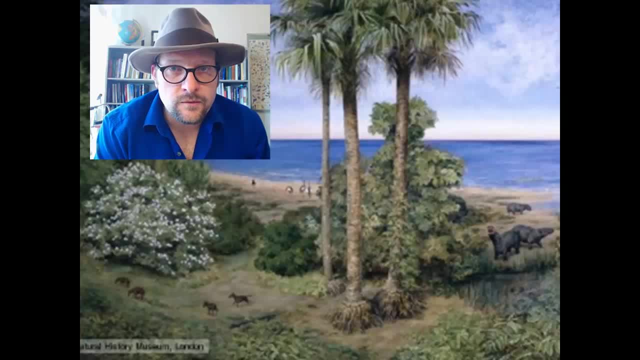 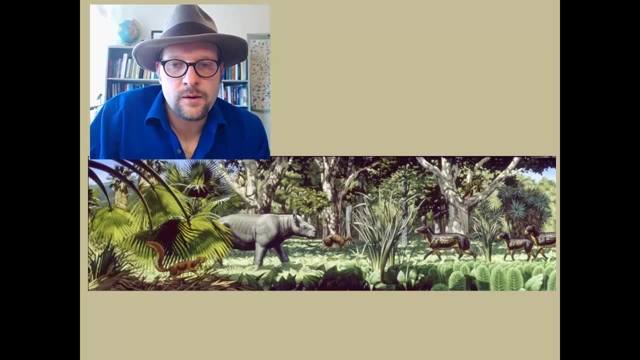 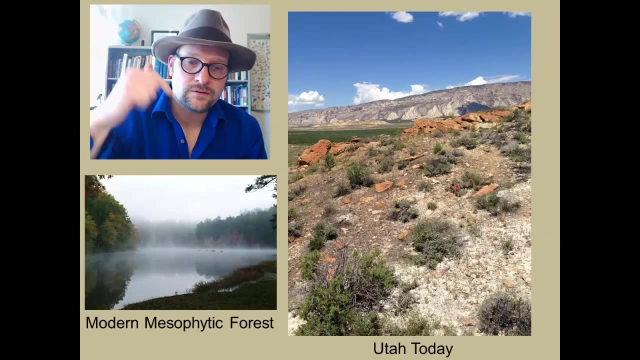 This is another reconstruction from the Natural History Museum of London of the Green River Formation during the Eocene period, And here is a reconstruction from the Smithsonian Institute in Washington DC. Comparing the environment of the mesophilic forests today with the modern northeastern Utah, it is striking how much the environment has changed during the last 50 million years. 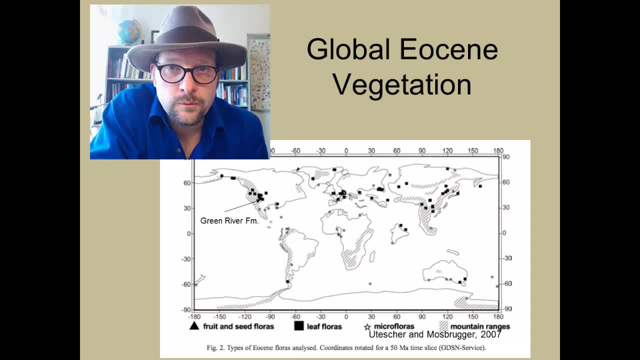 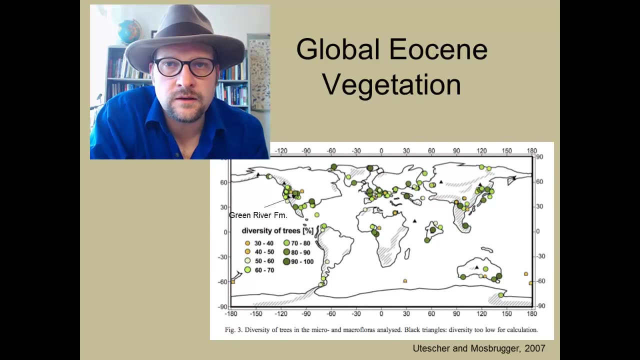 There are many fossil sites in the Eocene that preserve fossil plants from around the world, And it is interesting to get a global perspective on the middle Eocene biomes. if we compare these sites, One of the most compelling things is how diverse the flora is during the Eocene. 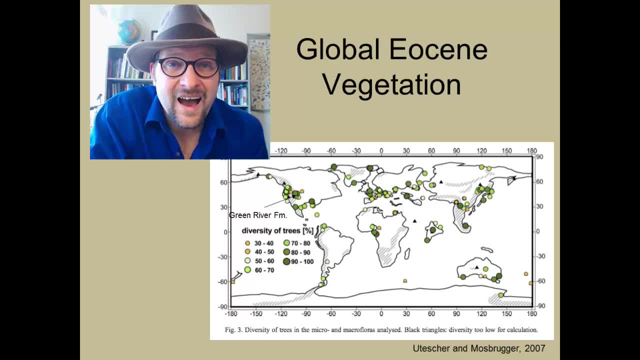 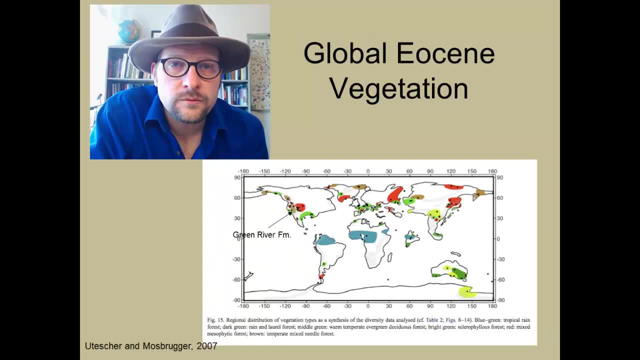 Even at high latitudes near the poles we see high diversity of plant life. so Utah was not alone in how warm it was. Reconstructing the Earth's biomes during the Eocene shows that North America was covered in thick rainforests to the south, mesophilic forests to the north. 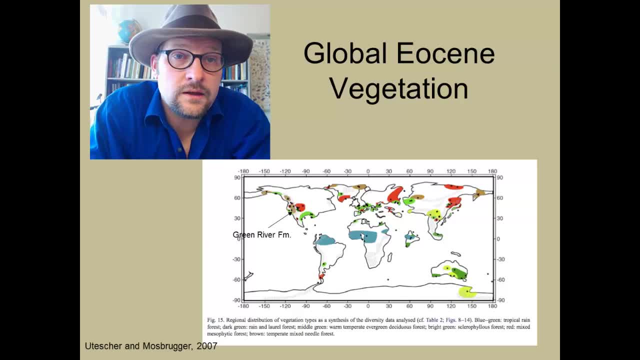 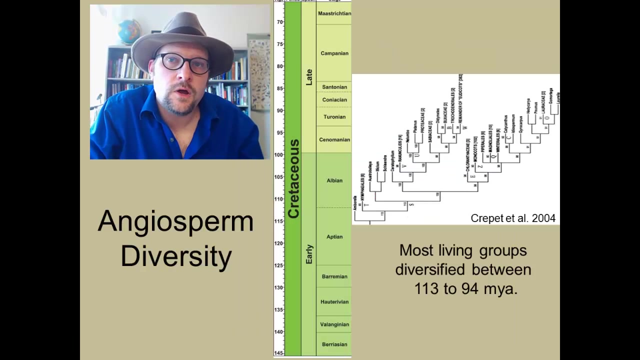 Hence it was as if the flora was shifting northward and much wetter and more temperate than today. The world was covered in a thick layer of forests and supported an extremely diverse fauna of animals. unlike anything we observe today, Much of the diversity of plant life was brought about during the Cretaceous. with that dramatic 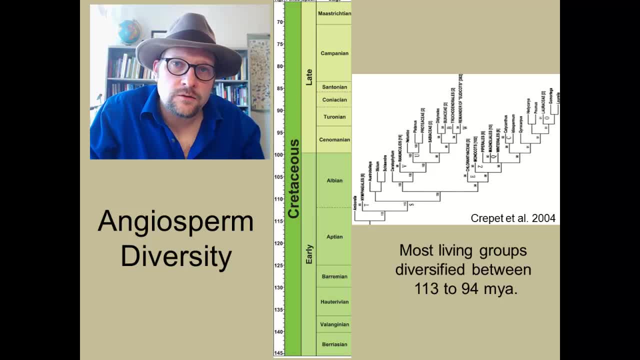 rise of the angiosperms. the flowering plants. The plants were dominated by flowering trees and shrubs and other. 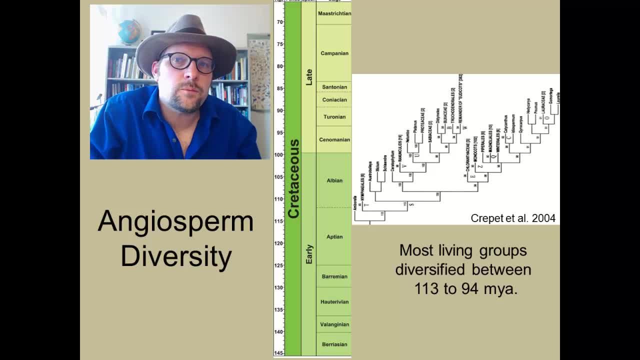 plants belonging to this new group. Not since the Pennsylvanian had seen earth in such floral diversity. these late Cretaceous and Eocene forests form a second pulse of coal-bearing. clásy DC units, And much of the coal in the western part of the United States comes from the dense flora. 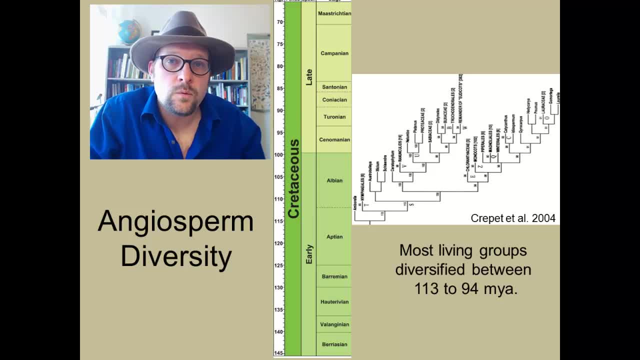 that lived during the late Cretaceous and up to the Eocene.